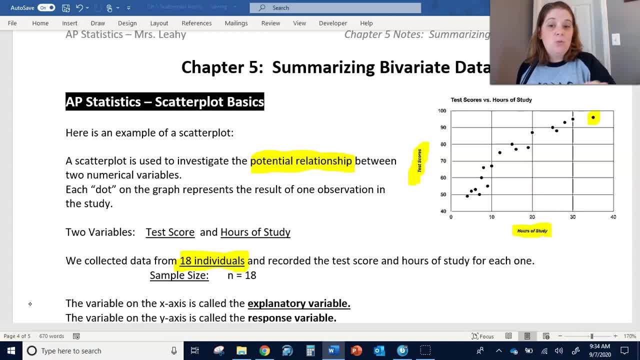 there are 18 dots. So we can tell that there were 18 individuals that were asked these two questions. So we can tell that there were 18 individuals that were asked these two questions. Remember, the variable is the question that was asked. So we can tell, because there are 18 dots. 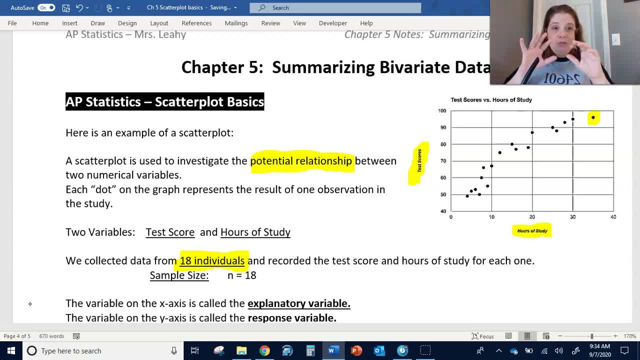 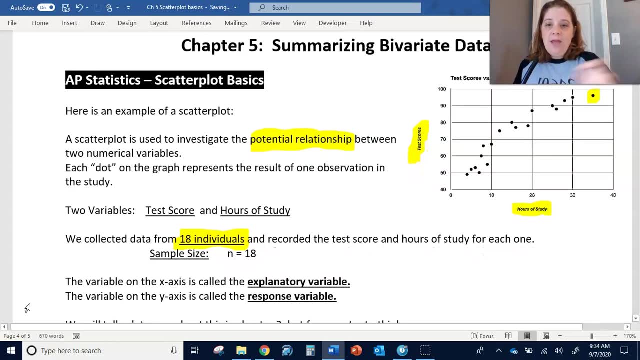 there was a sample size of 18.. Okay, so the sample size is the number of individuals, not the number of numbers. Okay, so we actually collected 36 numbers, but each set of ordered pair, each set of data, belongs to one individual. All right, so vocabulary here. 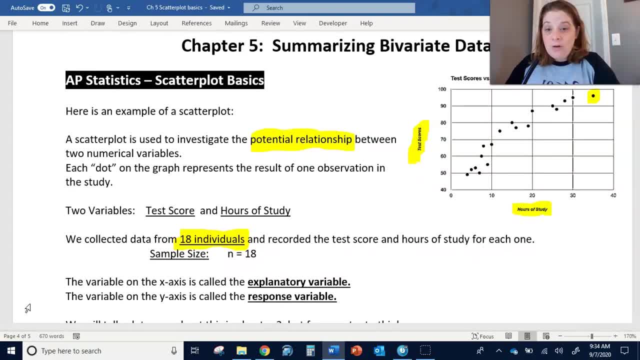 the variable on the x-axis is called the explanatory variable and the variable on the y-axis is called the response variable. Now, for right now, this is something that you can just memorize. We're going to be using this quite a bit in chapter two when we talk about experiment. 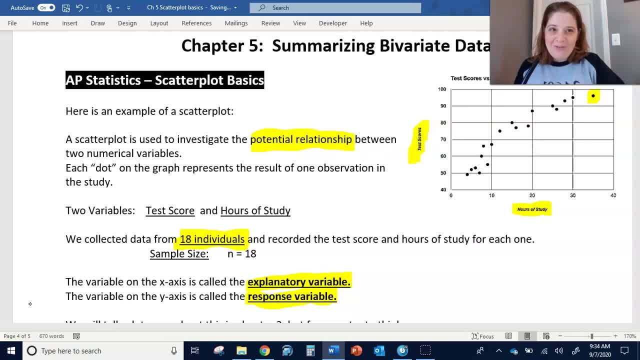 design, But in this case the explanatory variable is the one on the x-axis, Okay, and that's the one that we're trying to use to explain what's happening with the response variable. So we think there might be a relationship between how many hours you study and your test score, And so we're 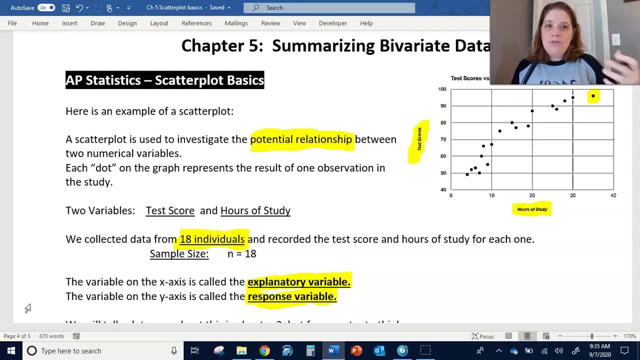 saying: as x changes the number of hours you study, the number of hours you study, the number of hours changes as the hours of study increases. what seems to be happening to test scores? Can we use hours of study to explain what's happening to test scores? Okay, so a lot of times we're going. 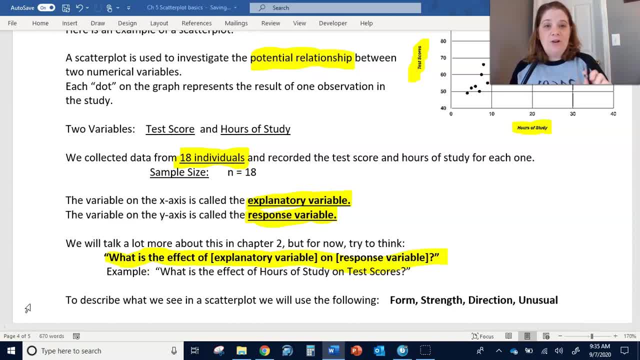 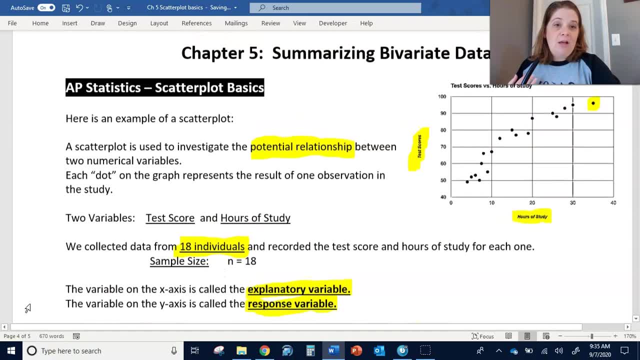 to have this statement. what is the effect of the explanatory variable on the response variable? What is the effect of hours of study on test scores? Now, to describe what we see in a scatter plot like this one up here in the right-hand corner of your notes, we're going to use four. 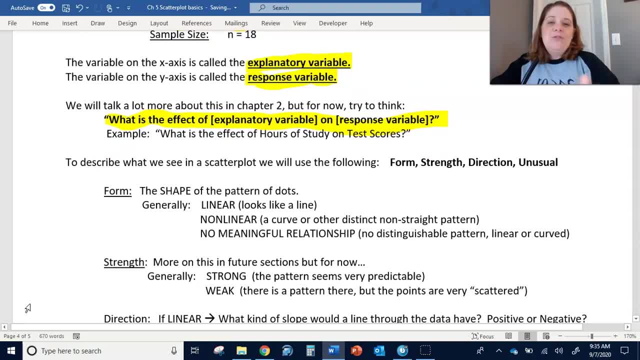 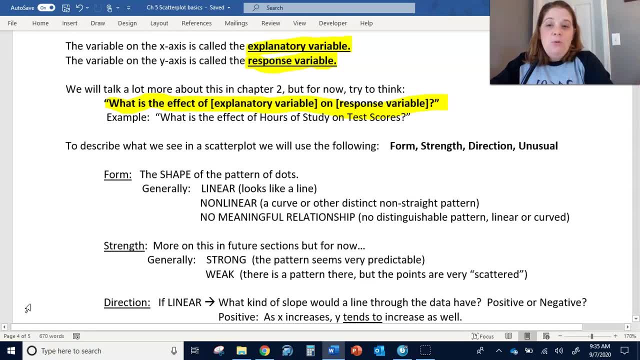 things. It's kind of like socks, but it's four, So we're going to be talking about form, strength, direction and anything unusual. Okay, so form is the shape Form. basically, we're saying: does this data look linear? Does it look kind of line-like? 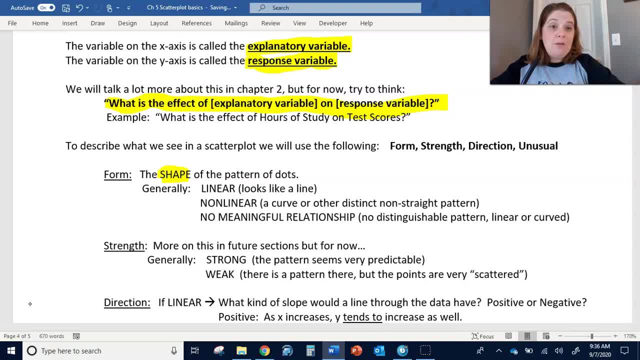 Does it look non-linear? Is it a curve, like a parabola or an exponential graph? Or is there no meaningful pattern, no meaningful relationship? Strength tells us how predictable the pattern is. A strong pattern means you have a very strong inclination about where those points are going. 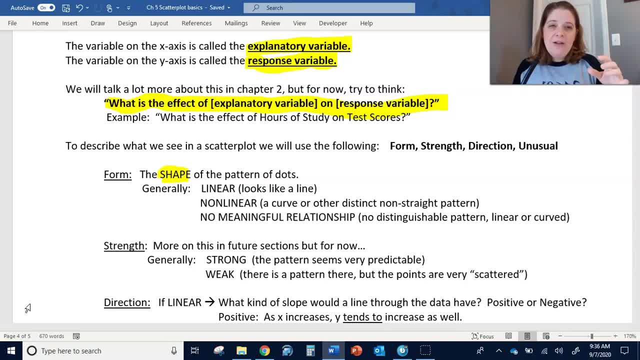 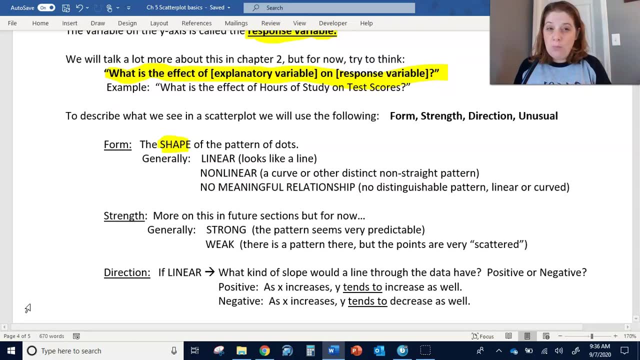 and you feel like you could make predictions. Weak means that there's a pattern there, but not very. it's pretty scattered. There's not a lot of predictability in what's going on. And then direction: if it is linear, we like to say what's happening as x increases or we're going to slope. 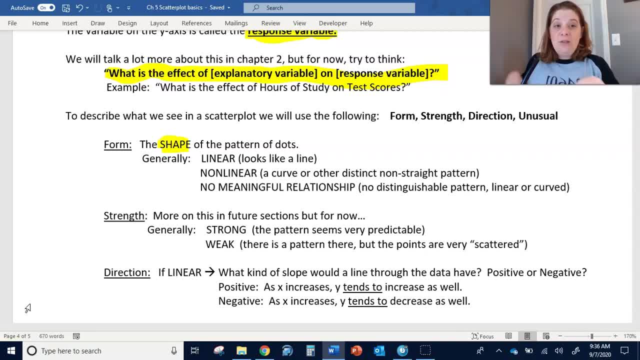 with this half. So we're talking about the rise over run of the line of best fit that would run through this. Is it going to be positive or negative? Is it going to be negative or negative? There is a phrase that you're going to want big time for weaseling in this chapter. It's the word. 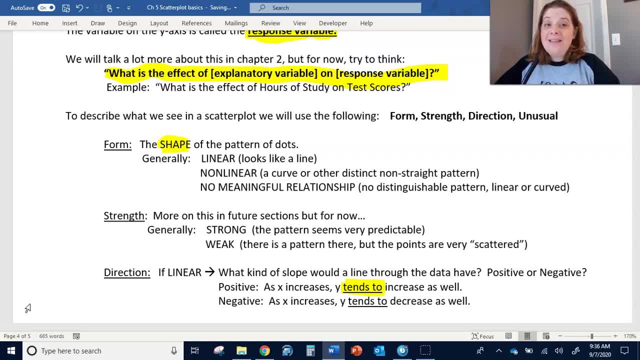 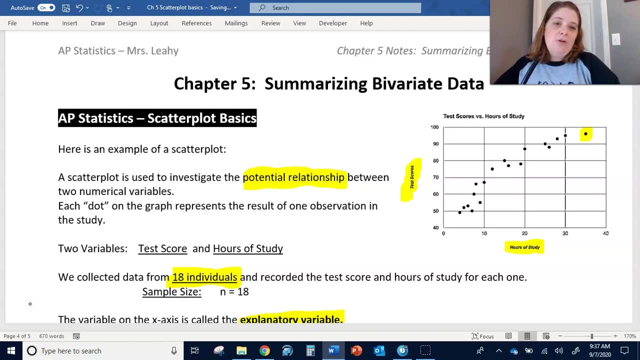 tends to. So a positive slope is one where, as x increases, y tends to increase as well. As x increases, y tends to decrease as well. So I'm going to go back up to my picture up here in the corner. So what I notice is that this might be curving slightly, but for the most part, I think. 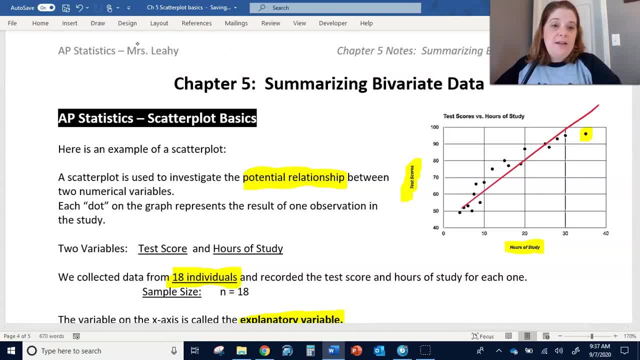 that this looks fairly linear. Okay, so I think that it seems to be curving slightly, but for the most part, I think that it seems to be following sort of a line-like pattern, although you might argue that it is doing some sort of curve here. It's relatively strong and it looks like it's. 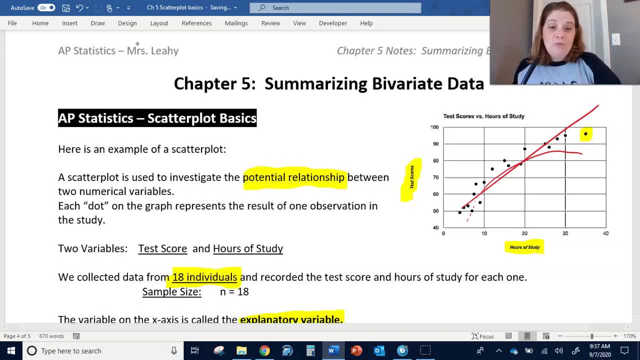 positive. As x increases, as hours of study increases, it looks like y tends to increase as well. Now again, the reason why we use the word tends to, instead of just as x increases, y increases, is because this is not a straight line And when I look at, say these two points right here. 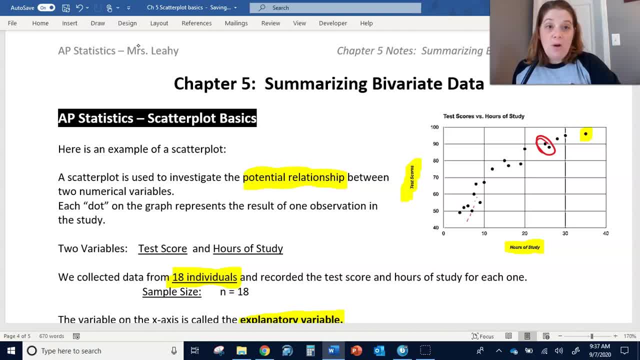 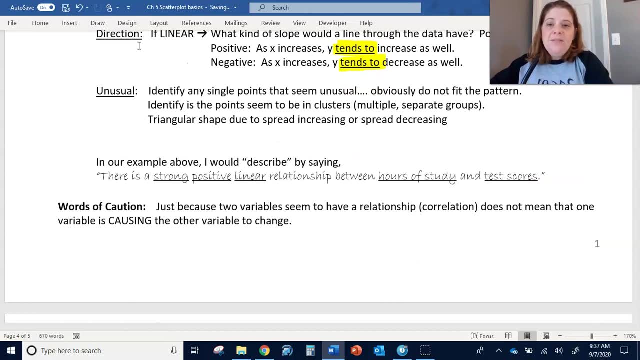 the one on the right has a bigger x value but a smaller x value. So I'm going to go back up to my smaller y value. So that's a case where, as x increases, y didn't increase. So we're talking about an overall behavior, a tends to, rather than just the value there. So again, in this example, 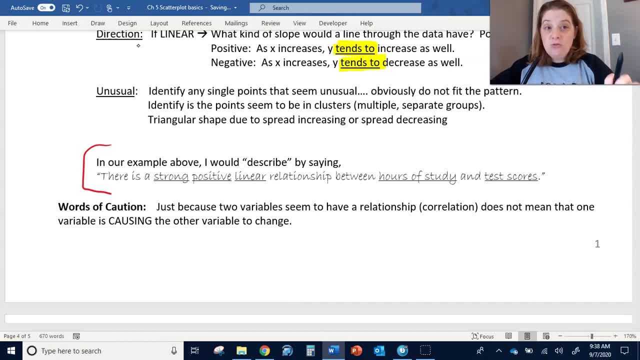 if I was asked to describe, I would say there is a strong, positive linear relationship. So here's my form: linear, Here's my direction. positive, Here's my strength. strong between hours of study and test scores. So I'm always going to write my x variable. 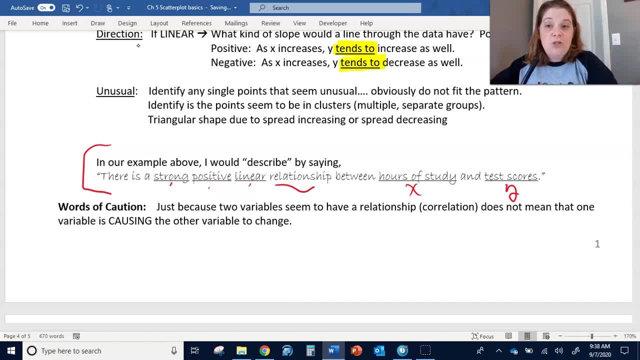 and my y variable in context to describe that relationship. Now, another thing we tend to look for is anything unusual, points that don't fit the pattern- And we're going to talk about those more in section 5.3.. But we want to identify things that don't look like they fit the pattern of the. 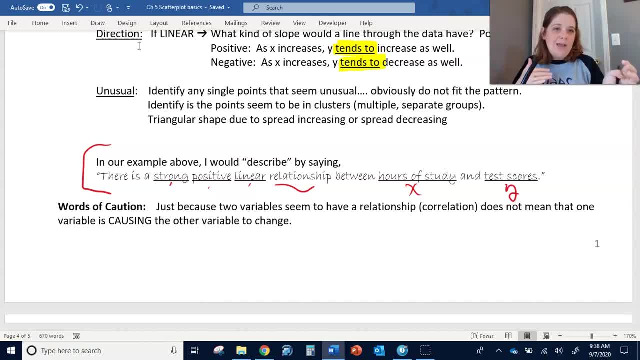 points Does it not seem to follow. Is it way out there to the side? Is it way out there above or below? And then we're going to look at the points that don't fit the pattern of the points. So we're going to look at the points that don't fit the pattern of the points. Is it way out there to the side? Is it way out there above or below? 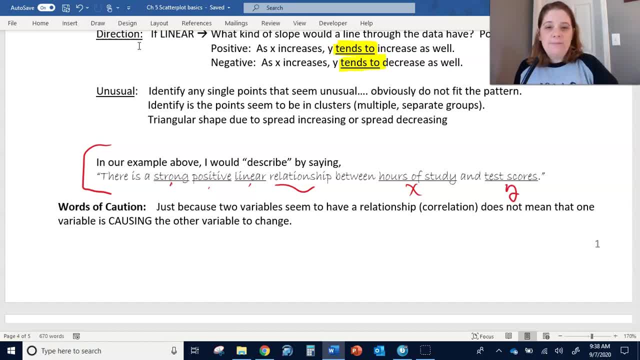 Is there a cluster? Is there a gap? We always want to look out for things that seem interesting. All right now. big word of caution: Just because two variables seem to have a relationship doesn't mean that one variable is causing the other one to change. So in our case, just because 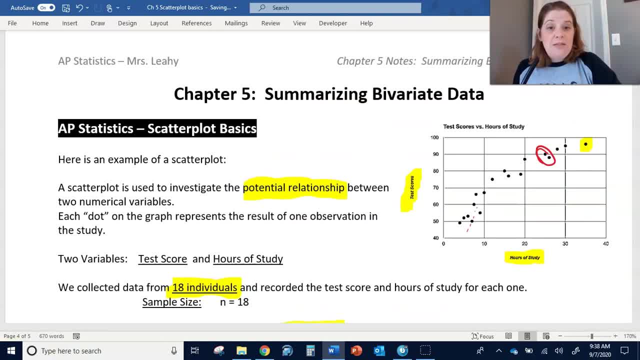 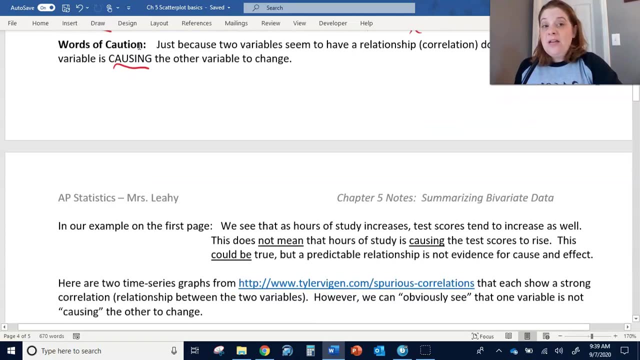 it looks like the more hours you study, the higher your test grade would be does not mean that the hours of study are causing the test scores to be higher. We have to be very careful about the way we word that. There could be some other underlying thing there that people who studied for longer maybe also did. 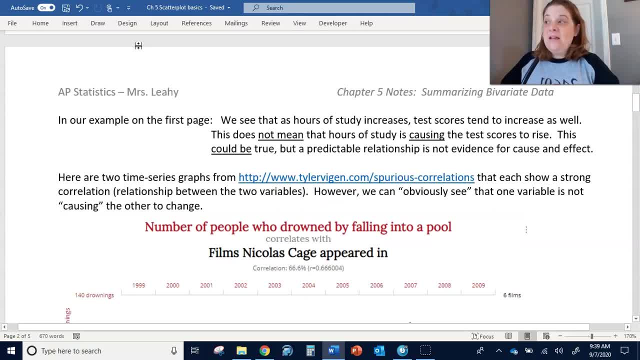 more homework, or people who studied for longer, maybe they have a better understanding, or something like that. I mean, there could be something else going on there. Okay, so in our first page again, just because we see that hours of study increases, test scores tend to increase as well. that doesn't. 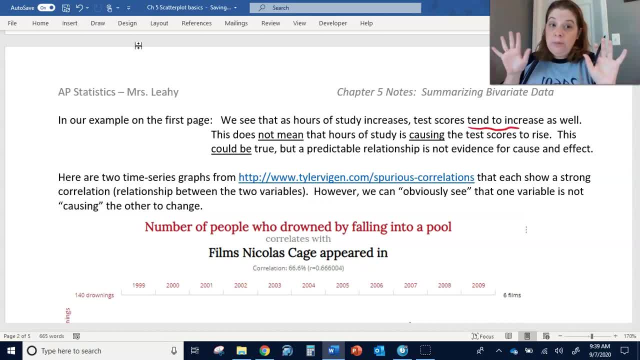 mean that one is causing the other to rise. It could be true, Could be Okay, but when we talk about a predictable relationship, we're not talking about a predictable relationship. We're not talking about a predictable relationship relationship. we're not talking about cause and effect. okay, so we're not. these are not cause and 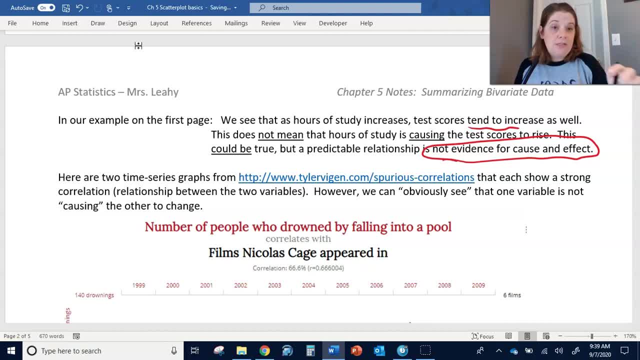 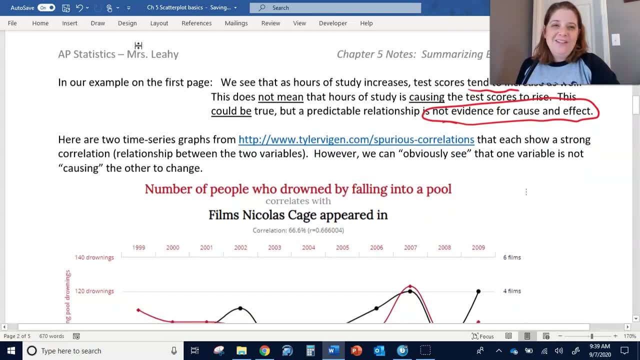 effect graph. this is increasing because the other thing is increasing or decreasing. um, we're just talking about a relationship that can help us to make predictions. okay, and just to kind of illustrate this a little bit, there is a guy named tyler vegan who has a whole study of these relationships that 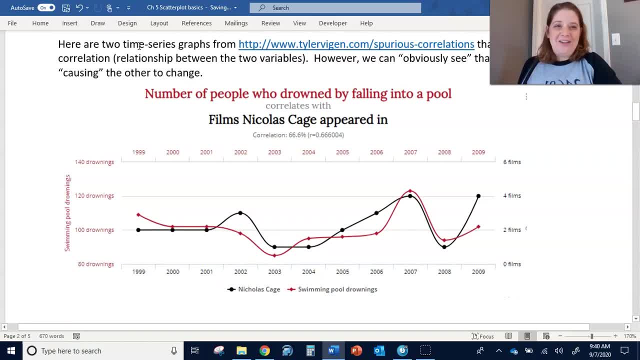 have a very strong correlation, but they don't actually have anything to do. so this is the number of people who drowned by falling in a pool, followed by the films nicholas cage appeared in in each year. okay, so you can see that these two things seem to correlate very well. there seems to. 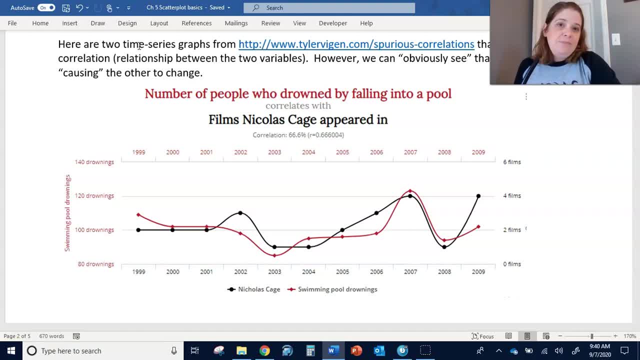 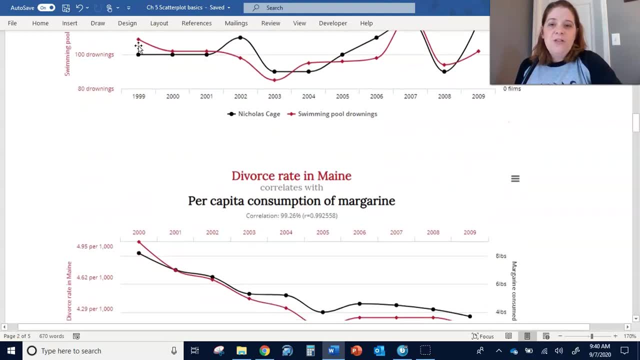 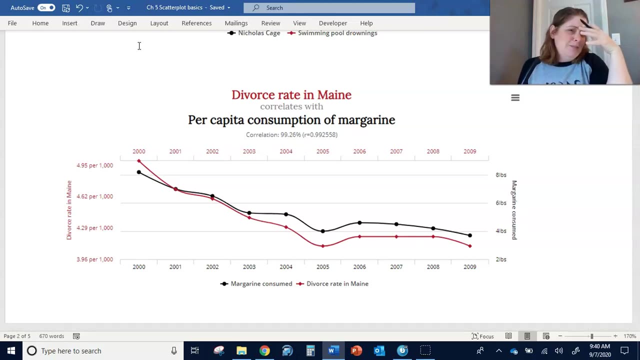 be a very strong relationship, but that doesn't mean that, as the number of people who drown in a pool increases, that nicholas cage gets to be in more movies. okay, here's another one. this is the divorce rate in maine and the per capita consumption of margarine. right, like i can't believe it wasn't. 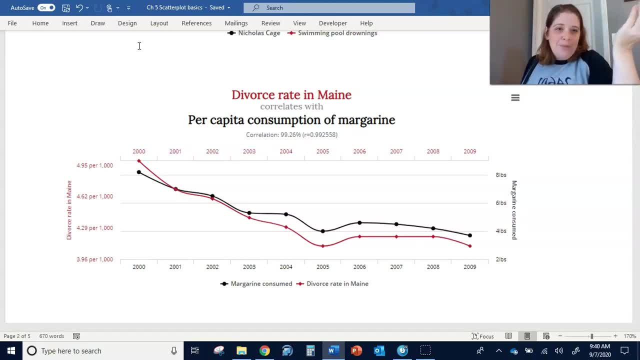 butter, right, i mean like it, the, the, the. the butter is not causing the margarine's, not causing the divorce rate to to fall or rise for each of these years. so sometimes you'll see relationships between two things, and just because there's a relationship does not mean there's any sort of cause happening there. all right, so if you 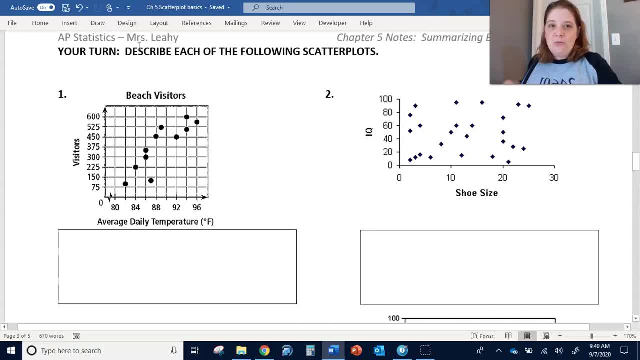 were going to describe each of these scatter plots. again, we're looking for that direction: unusual form and strength. so i'm going to take a look at this and let's see, it looks like this is, in general, increasing. here i've got my two variables, so i'm going to type into this link. i'm going to say there: 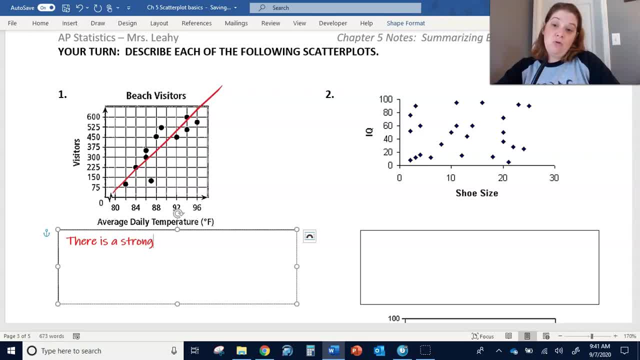 is a strong because it looks pretty predictable. if i went over to 97 or 98 i have a pretty good idea of what's going on there. a strong positive because the slope of that line is positive. linear relationship- oh, i can't spell relationship between visitors or, sorry, between average daily temperature. 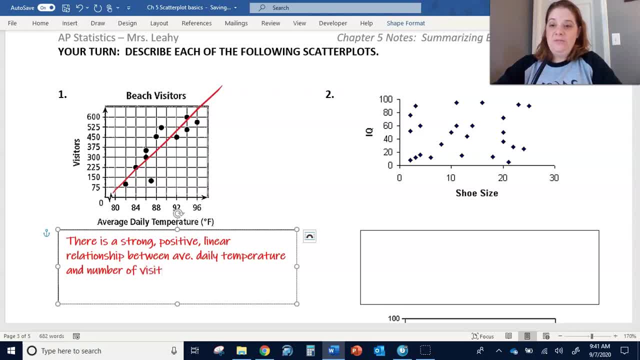 and number of visitors. there's a strong positive linear relationship between my two variables over here. i look at this. i've got iq and shoe size. i don't think this is positive or negative. that just seems to be very randomly scattered. so i'm just going to say 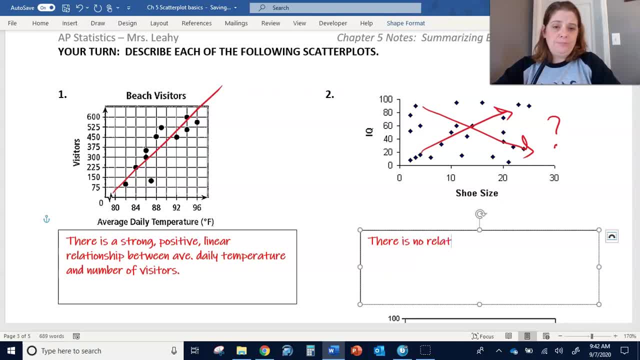 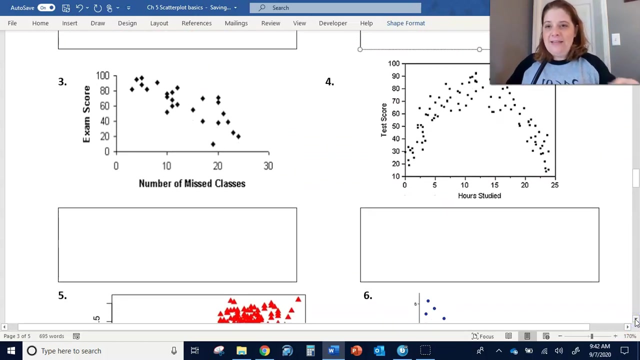 there is no relationship- or actually i'm going to throw in another word, there's no meaningful relationship here- Relationship between shoe size and IQ. So I cannot tell, based on your shoe size, whether or not you will be more or less intelligent. All right, number of missed classes and exam score Okay. 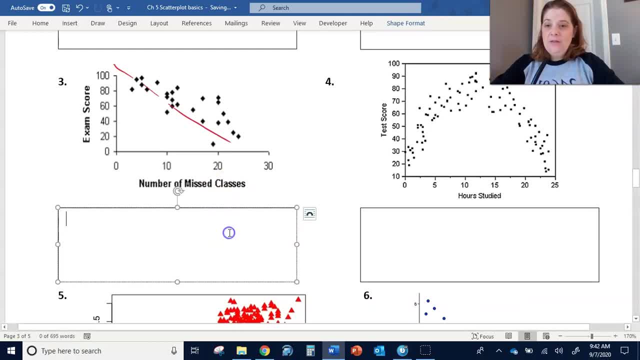 so again, I look sort of like a negative line here. Okay, so I would say there is a- and that's fairly predictable- strong negative linear relationship between number of missed classes and exam score. Okay, and then over here: wow, now this looks to me like a parabola, like very, very strong, but I mean. 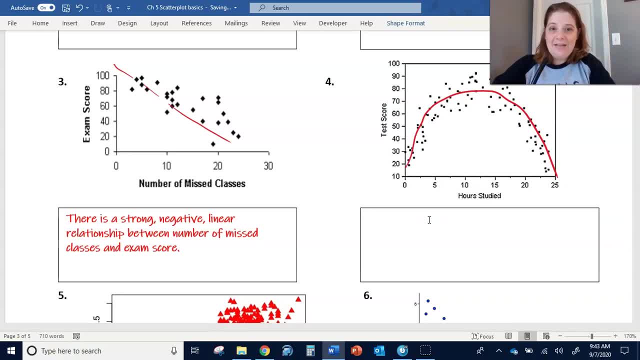 so it's definitely there's a strong something happening here, but it is not a line, Okay. so I'm going to say there is a strong non-linear- if you want to, you could say curved- relationship between hours studied and test score. Okay, so notice that I didn't say positive or negative, because this is curved And so 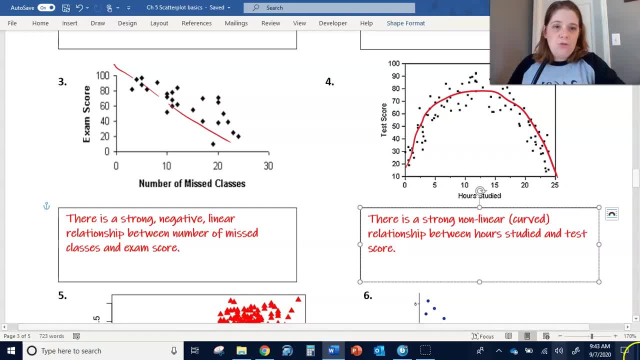 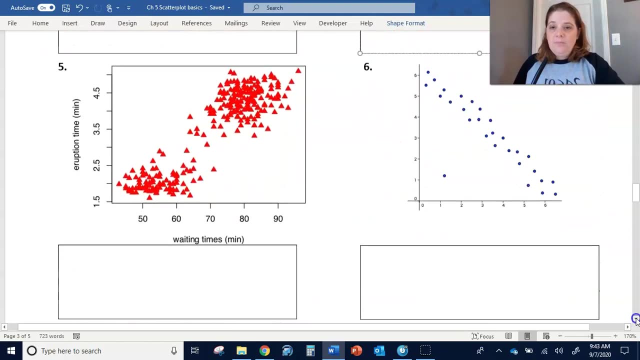 if something's linear, it's going to have slope, but otherwise we're not going to describe that. Now you could say something like: the scores increase until about 12 hours and they start to decrease, But that's. that is a non-linear relationship here. Okay, now here is. 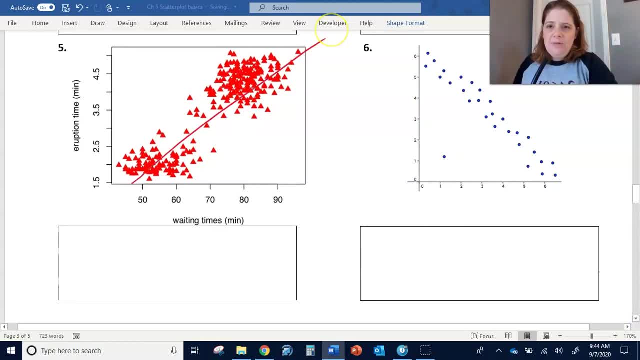 another kind of interesting thing that I want to talk about here. So I'm going to say okay. so I'm going to say okay, so there is a okay, so definitely not strong. So I'm going to say, um, I'm going to say weak, positive, linear relationship. 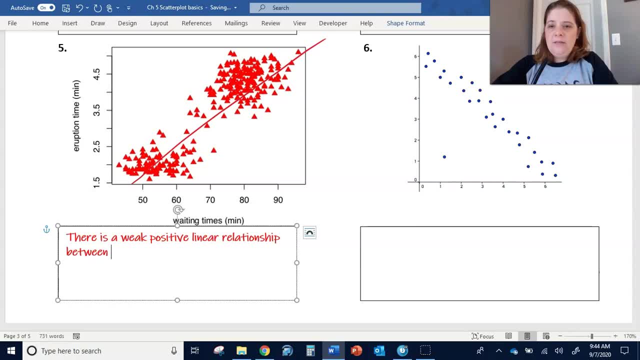 between waiting times and eruption time. Um, I'm going to also say also: it appears there are two clusters of points Um, one from zero to 70 minutes And waiting time, And a second from 70 to 90 minutes waiting time. 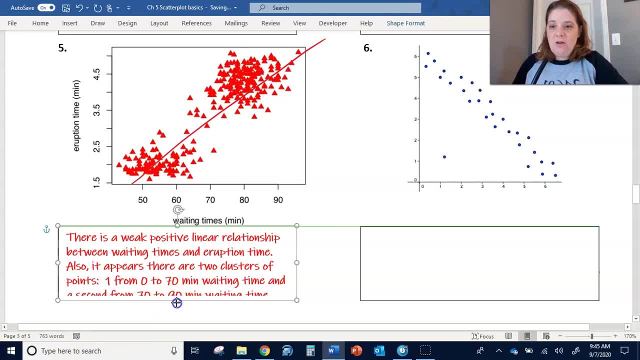 And I just started to write minutes, but that doesn't work because the other axis is also measured in minutes, So I have to be a little bit more specific. Okay, now this next one. I've got a definitely negative. It's very strong, But then there's like: what in the world is going on right here? 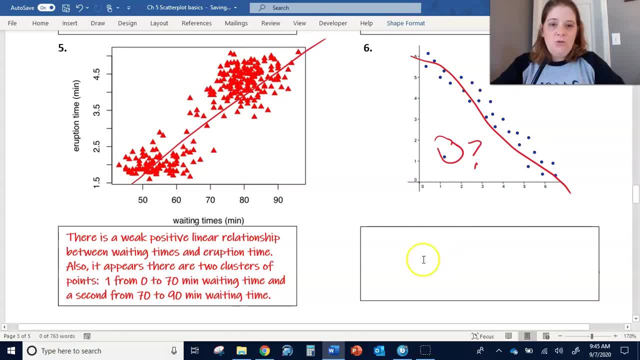 But then there's like what in the world is going on right here? But then there's like what in the world is going on right here? Okay, so wrong. it's going to go weird. in the next run I'm going to change if here. 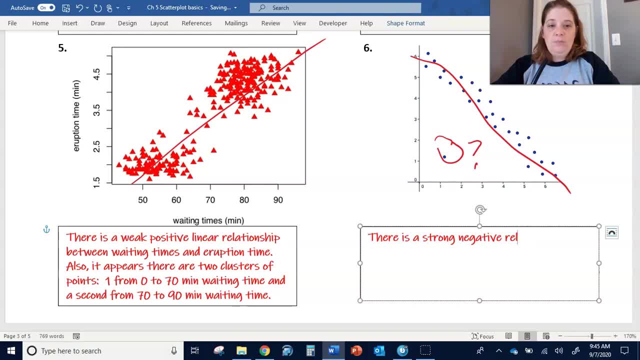 there's something that I need to ifty post this one. I'm going to add it because we thought we finished that and then change all of that again. Okay, let's come back here. Let's go back here, right here, to your calculator. 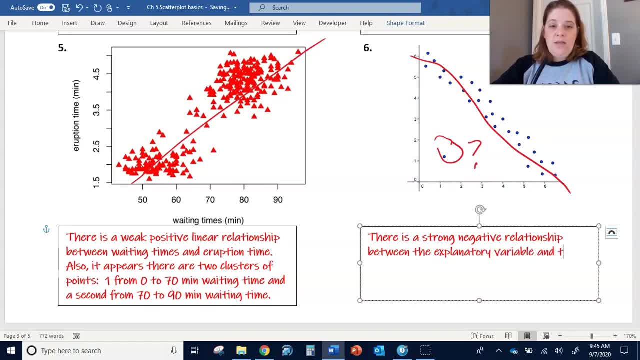 Great. And then let's come back here. Two points get the same, two gets the same, then something all get the same相: aşk right here. variable. okay, I really want context on those, but I don't have any, so I'm going to use this instead. 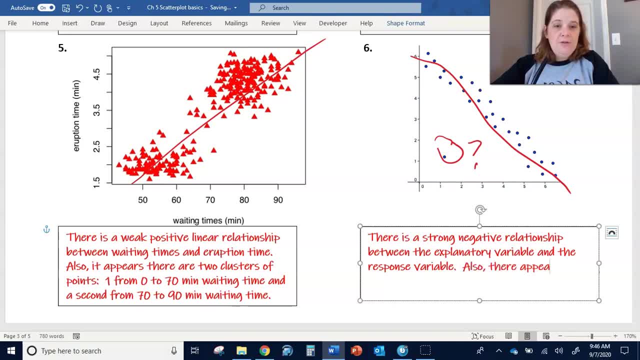 also, there appears to be an outlier at about 1.5- 1.5. so I don't know specifically if there's going to what these variables are, or what this or but- and we're going to talk more about outliers later, but that point just doesn't seem to fit the pattern. 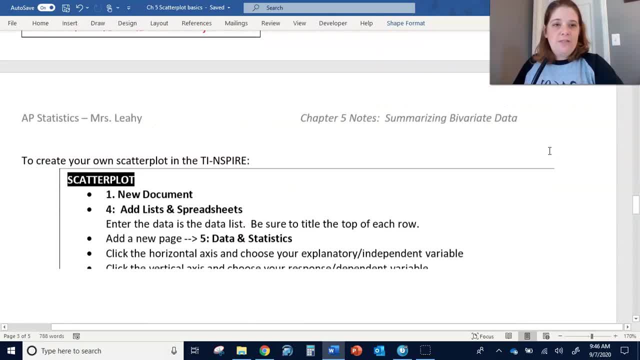 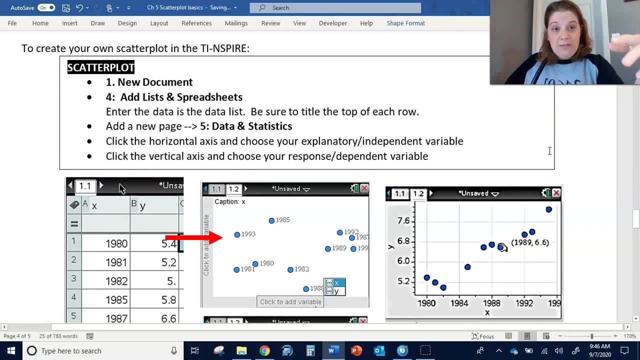 all right, so I'm going to describe those. oh, and I just flipped that over. that's exciting. okay, now to use your TI Inspire to make a scatter plot. you're going to do the same thing you did with one variable data, in that you're going to put everything in a list. but now you're going to 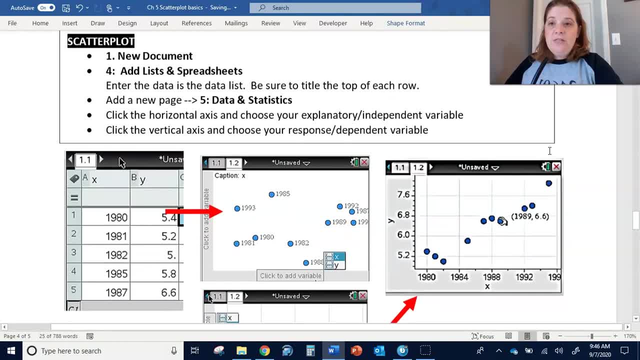 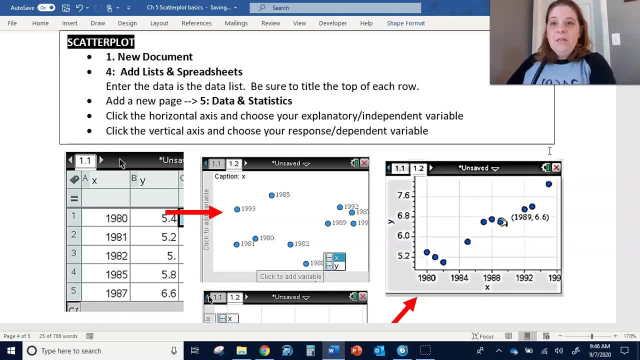 write them as ordered pairs in two lists. okay, now here's an example of kind of what I've done on your paper, so you can follow along. okay, so you're going to make a list with x and a list with y, okay, and your list and spreadsheet, and then you'll add that new data and statistics page. 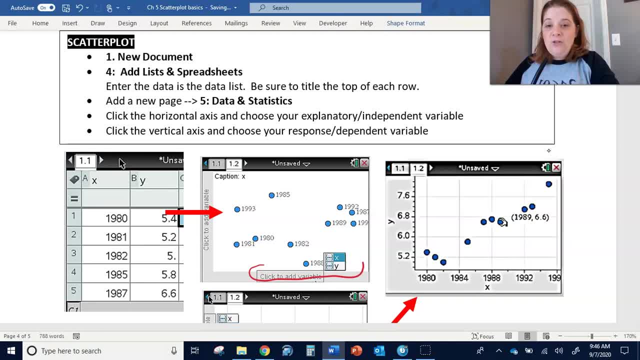 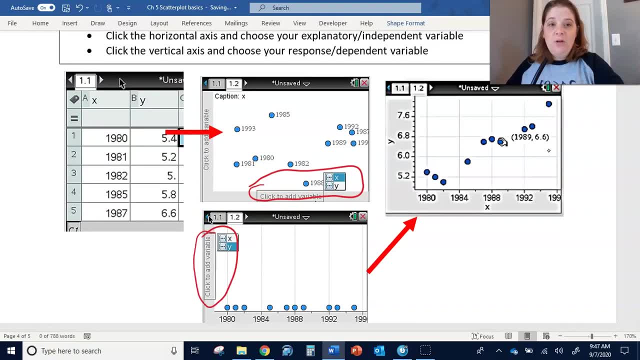 on the x-axis, you will click and add your x variable, and then on your y-axis, you will click and add your y variable. that's going to give you this delightful little scatter plot. and then, if I wanted to transfer this onto my paper, I would just mimic the scale that was given to me and then I would. 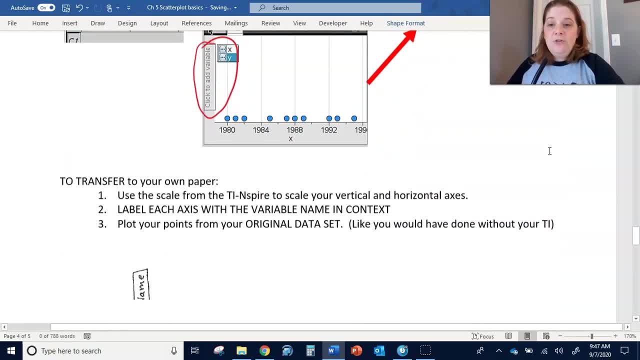 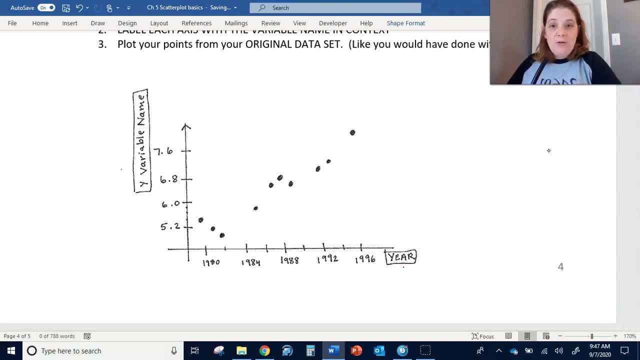 literally just plot the points. okay, so down here to transfer that onto my paper, I would mimic the scale, I'd make sure I labeled my both axes here, and then I would take my points from my original data set, like I would have done without my TI, and plot the points where I was there. okay, so it's a really quick way in order. 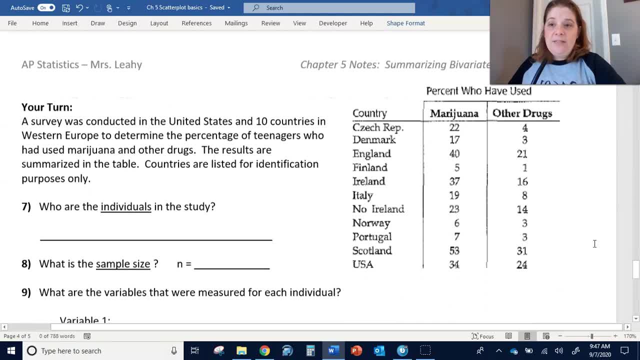 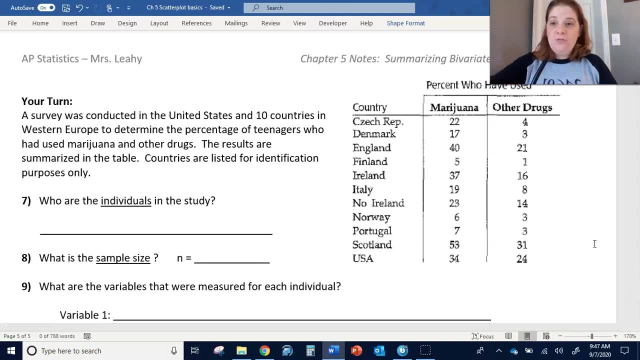 to do that, all right. so here we have an example and it says a survey was conducted in the United States and 10 countries in Western Europe to determine the percentage of teenagers who had used marijuana and other drugs. the results are summarized in the table. countries are used for. 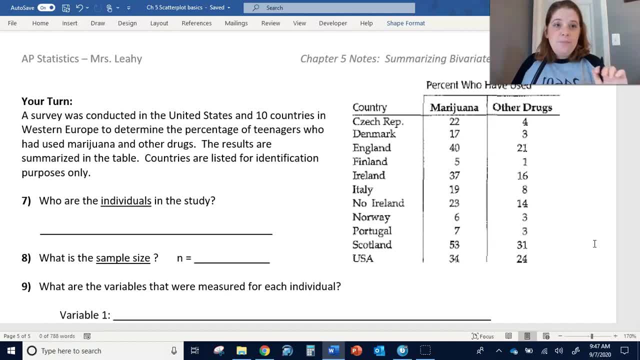 identification purposes only, all right. so this is something that some people have been having struggle for. if I have this country over here, so to the Czech Republic, for example. in this example I've got marijuana and other drugs. this up here is an ordered pair that we're going to look at once. I've got that ordered. 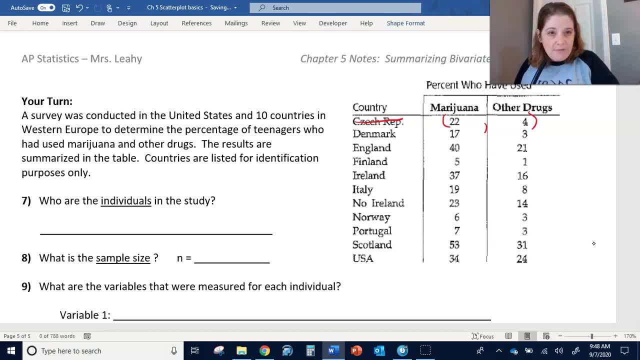 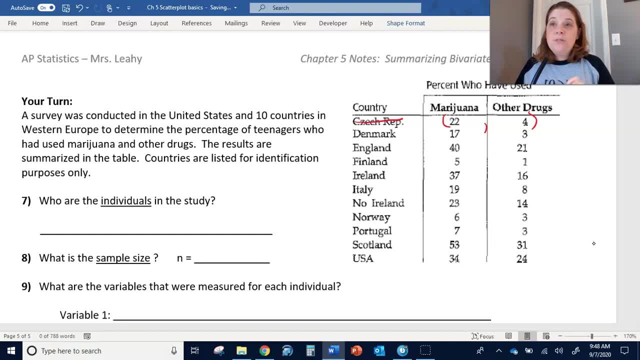 go ahead and write that down over here in the right hand corner. okay, so it says who are the individuals who went and asked the questions and it says what was the percentage of their data and even though we don't know the exact number right now, we're only going to go ahead and approximately the. 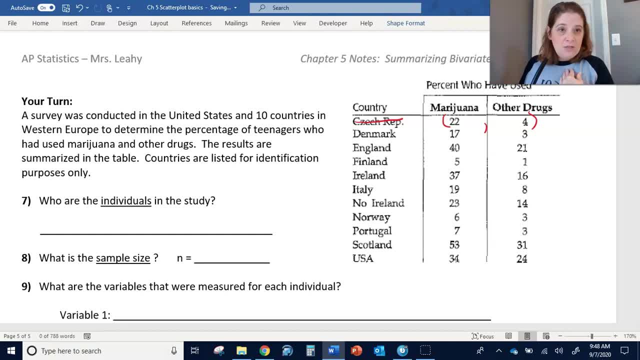 percentage of the data. we still have that recorded. we might use that later. there was an example about using boardwalk and park place and their prices. I don't need to include the words boardwalk and Park Place anywhere on my graph. okay, I'm just looking at the numerical data. okay, so it says who. 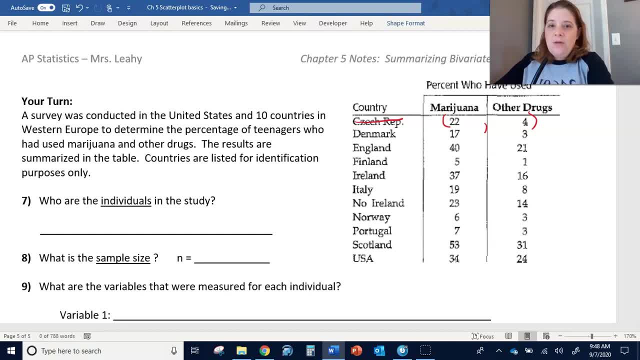 are the individuals in the study. so the individuals are the people. we went and asked the questions. okay, so in this case, the individuals are going to be the countries and there are 10 individuals out, 10 of these countries plus the United States, So there are 11 countries. So that gives me a. 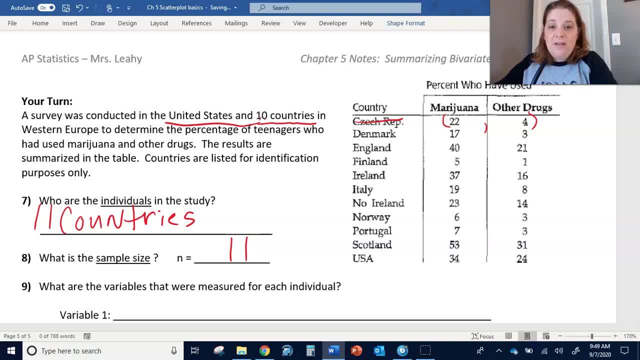 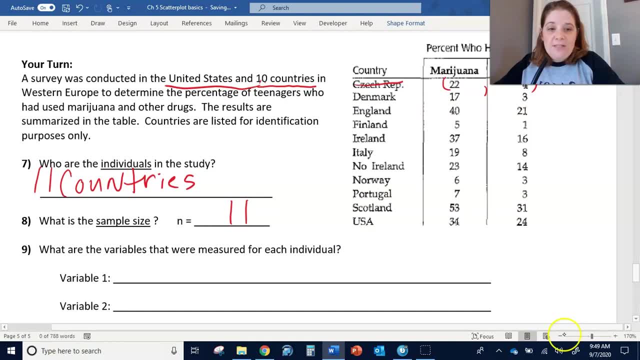 sample size of 11.. 1,, 2,, 3,, 4,, 5,, 6,, 7,, 8,, 9,, 10, 11.. It says what are the variables that were measured for each individual. Okay, so one thing I want to be careful of, because it's really 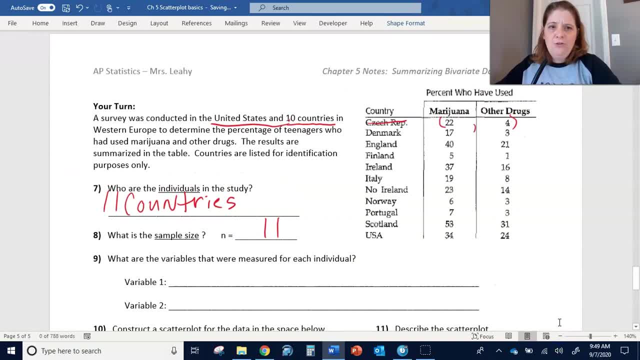 tempting here to write that my variables are marijuana and other drugs. but that's not a variable. A variable is not marijuana, That's not a variable. It has to be a question that you've asked. So this one, the first one we can say percent who have tried marijuana? 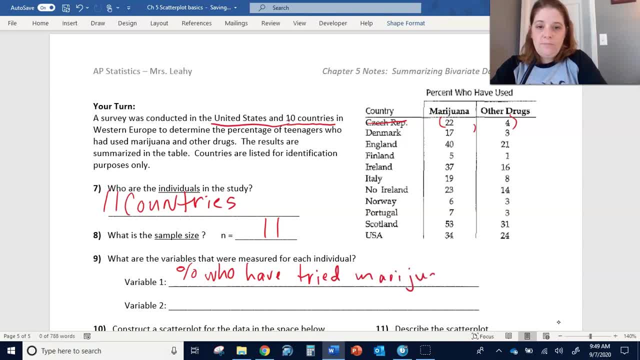 and percent who have tried other drugs. Okay. so we want to be careful. You don't just say marijuana and other drugs, because those are not variables, Those are just words, okay. So a variable has to imply that there's that could. 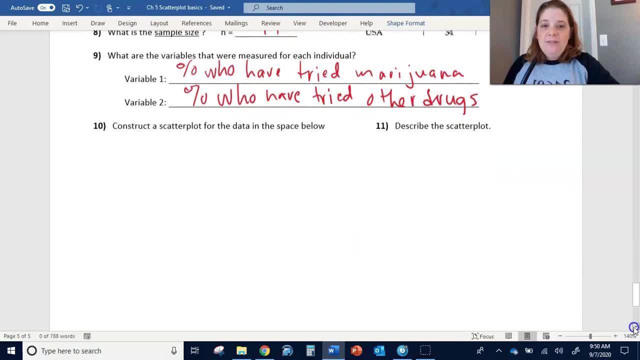 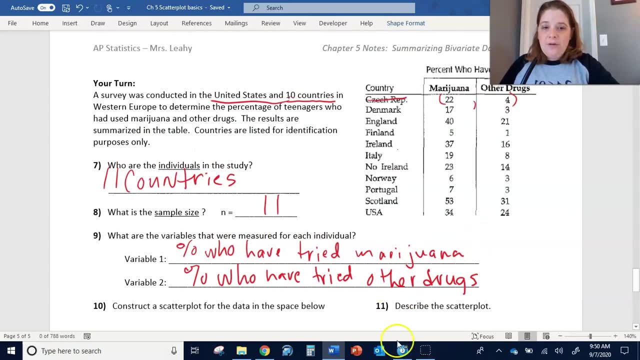 be changing, depend on who you ask. It says: construct a scatterplot in the space below and then describe the scatterplot. Okay, so I'm going to pause the video here and I'm going to open up my TI Inspire. okay, Actually, hold on. Here's my TI Inspire. I'm going to add a list and spreadsheet. 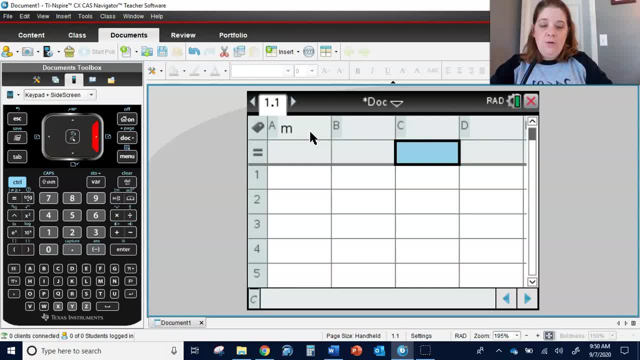 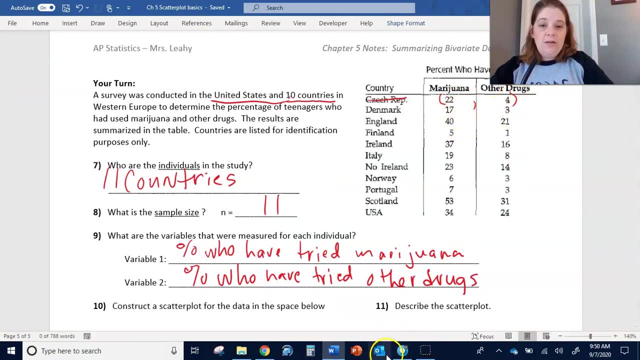 here and I'm going to put an M for marijuana And an O for other drugs And I'm going to type in so list and spreadsheet. I'm going to type in these values. So like the first one it goes 22 and 17 and 40, and this one is 4 and 3 and 21.. And 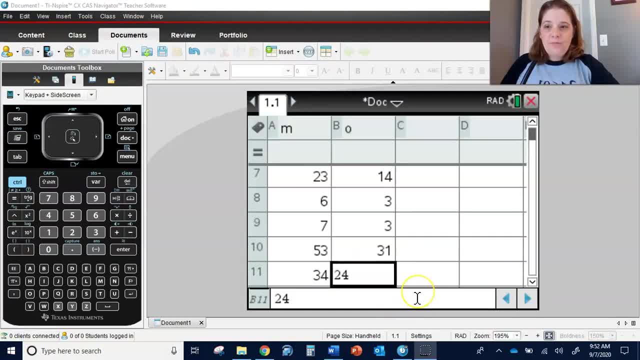 I'm going to type those in. So I'm going to pause the video. I'm going to type this data in. Okay, so I have taken this data and I have typed it in, So I have all of my percent. who tried? 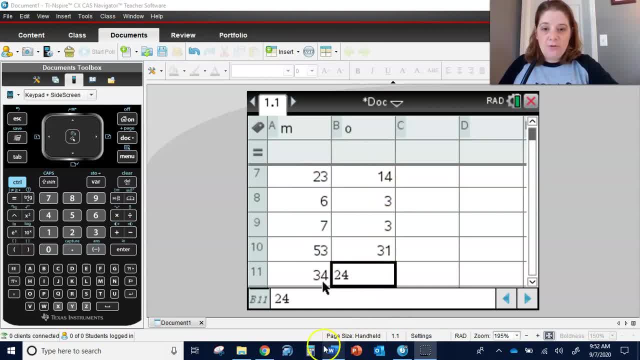 marijuana numbers in the first column and all of my percent who tried other drugs in the other column here, Okay, so I got those off of the table And I'm going to type in these values. Okay, notice, I have them labeled. Okay, the next thing I'm going to do is I'm going to create a new. 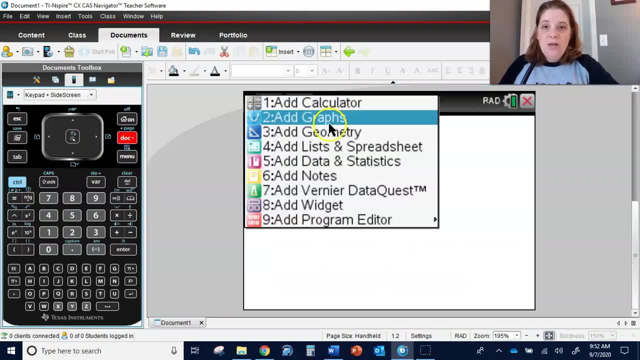 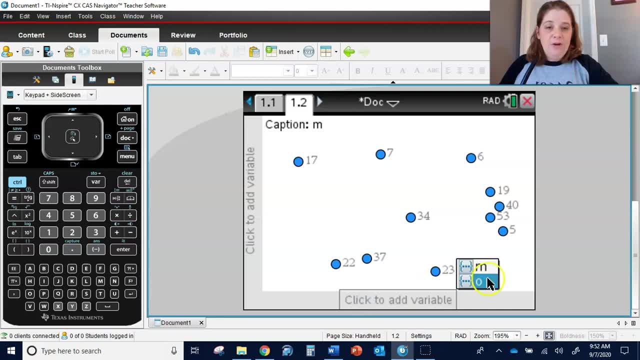 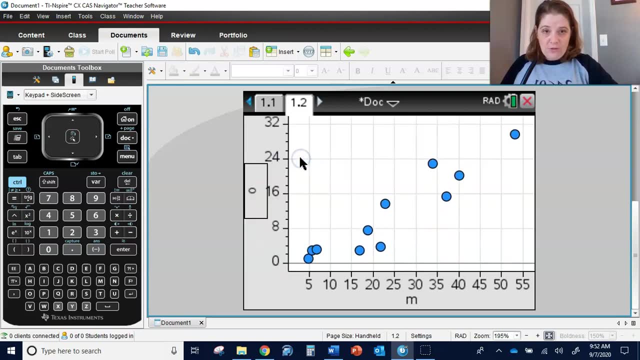 page. So I'm going to press control and dock to get a new page And we want a data and statistics page. I'm going to take my cursor down here, I'm going to click to add my variable, I'm going to put marijuana, That's my x-axis, And I'm going to click up here and I'm going to put O. There's. 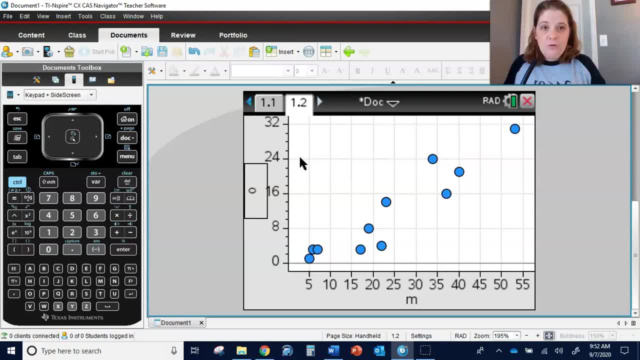 other drugs. And now I've got my other axis here. So notice that the graph goes 5,, 10,, 15,, 20,, 5,, 30, etc. It goes by 5s, from 5 up to 55.. And the other direction it's going from 0, and it's. 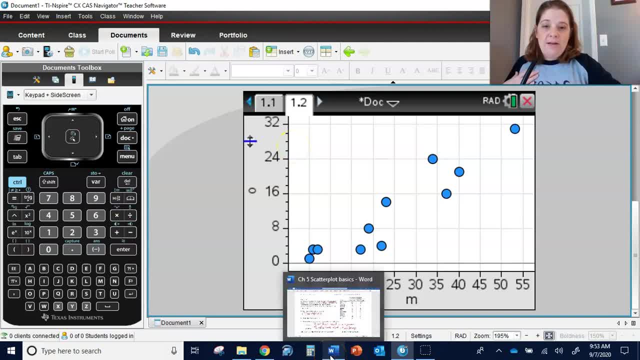 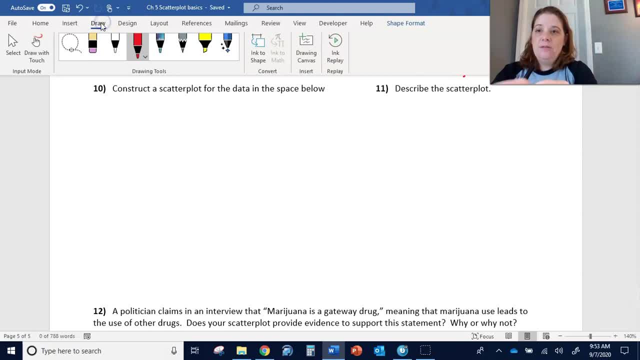 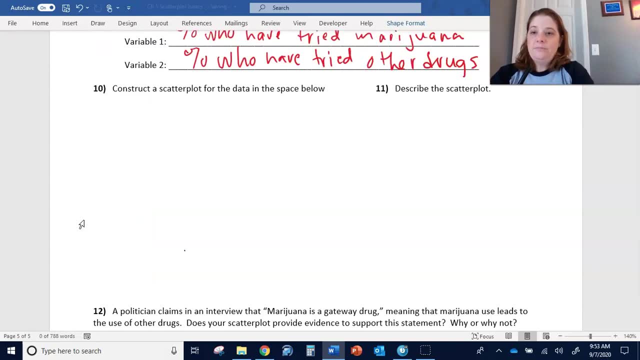 going by 8s up to 32.. So I'm just going to mimic that on my paper. So from 5 up to 55, and then from 0 up to 32 by 8s. Okay, so I'm going to take my handy dandy pen here. All right, so I'm going. 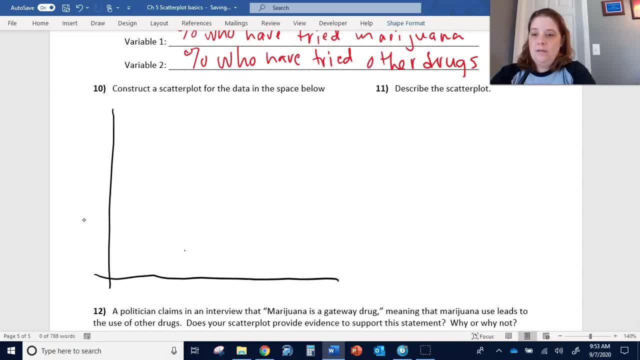 to draw this axis. Okay, and I've got 5,, 10,, 15,, 20,, 25,, 30,, 35,, 40,, 45,, 50,, 55.. Okay, and this is going to label the percent who've. 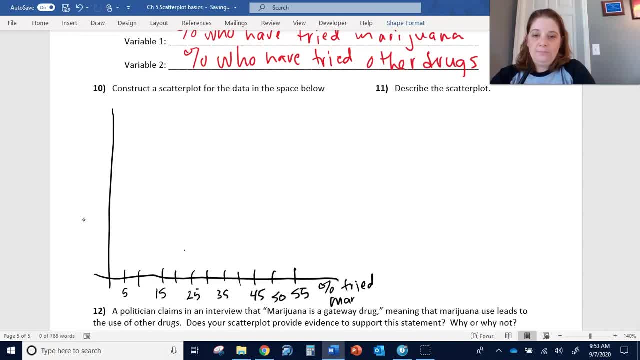 tried marijuana, And then I'm going to go the other direction and it went by 8s up to 32.. So 8, 10, 15,, 20,, 25,, 30,, 35,, 40,, 45,, 50,, 55. And this is going to label the percent who've tried. 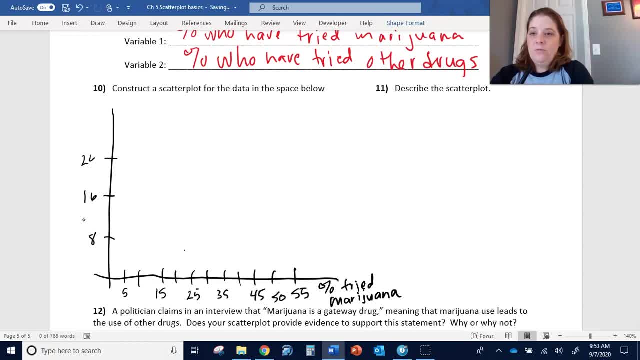 16,, 24, and 32.. And this is my percent. who've tried other drugs? Okay, so I've got those two labeled. I've got my axis. I just copied them pretty much straight off of that And now I'm. 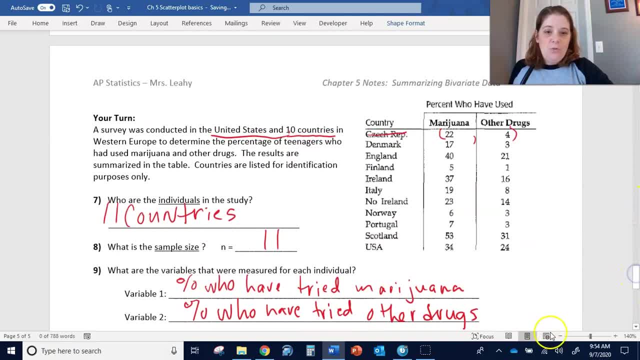 not going to go back to my calculator for this, because I've got this data. So my first point here was 22 and 4.. Okay, so I'm just going to zoom out so I can see it And I'm going to go. 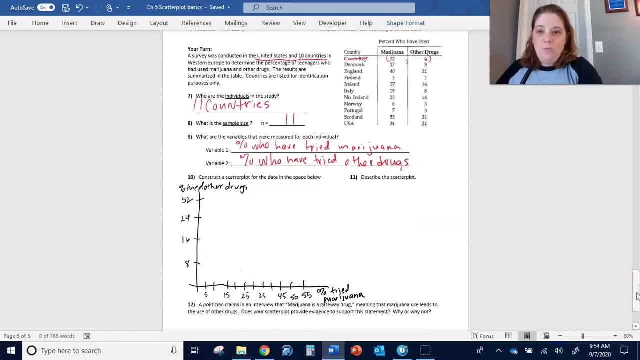 ahead and see all of this at once. So that 22 and 4, I'm just going to plot that where that would be. So here's 20,, 22, and 4, and 17, and 3.. Okay, so I'm just going to plot these points where they. 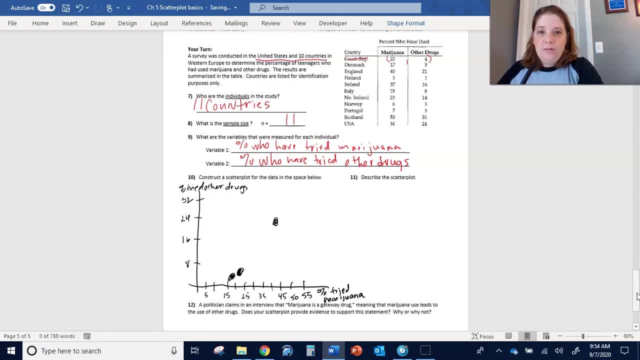 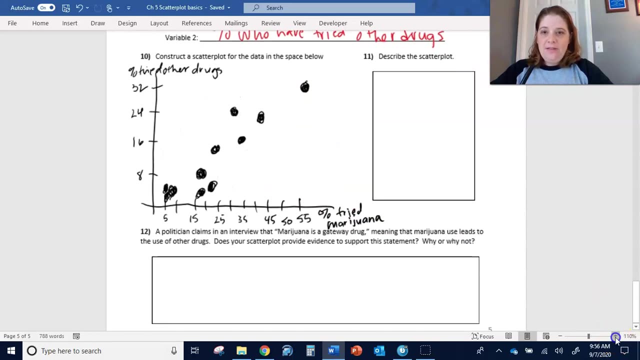 would go 40, and 21, and 5, and 1, and 37,, etc. All right, so I'm going to pause again and finish plotting those Transferred all of my points over here And you can see that I made my points kind of messy, Sorry. 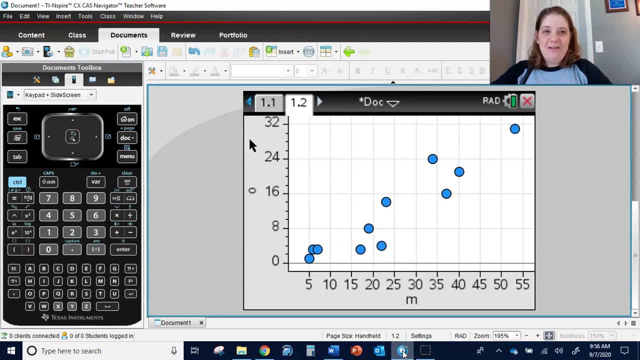 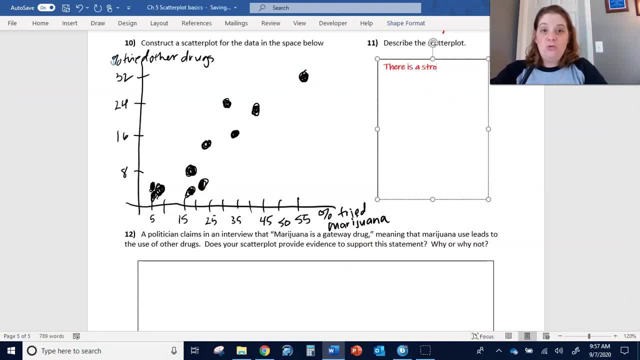 hard to draw on the screen. Hopefully yours are better. I just kind of have this appearance of the graph that was on our calculator here And if I was going to describe this then I would say it looks like there is a strong positive linear relationship between the percent. 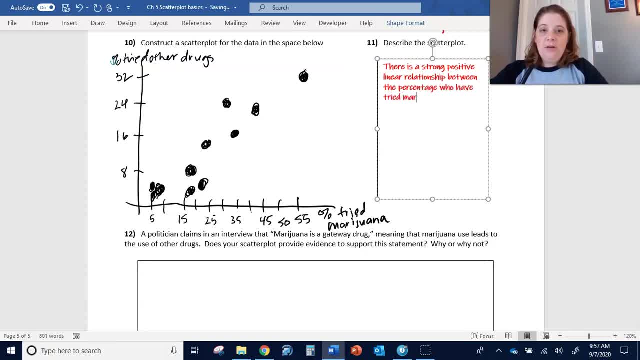 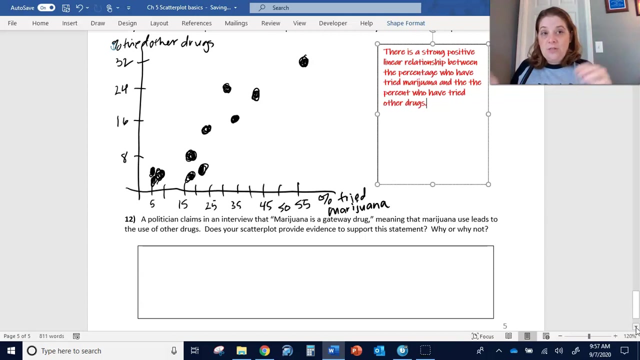 who have tried marijuana and the percent who have tried other drugs. I don't see anything unusual here, And so it does seem to be that, as the percentage in a country who tried marijuana tends to be higher, that the percent who have tried other drugs also seems to be higher, And so a 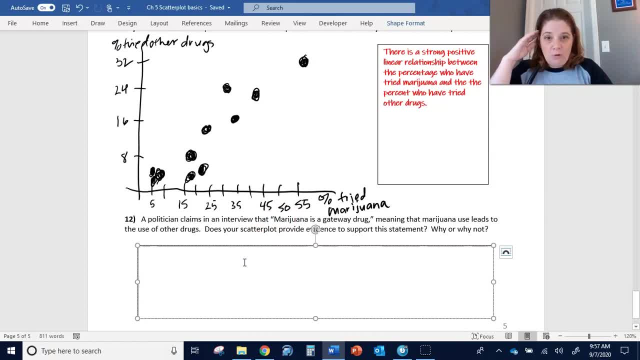 politician claims in an interview that marijuana is a good thing And he says: well, I don't know, gateway drug meaning that marijuana use leads to the use of other drugs. So what they're saying is if a person uses marijuana, they think, okay, marijuana is not that harmful, or whatever. 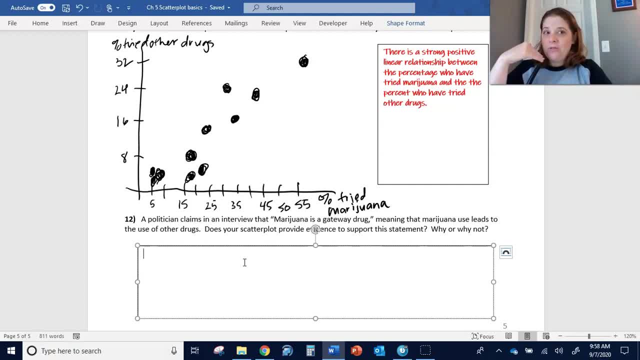 Does that make a person more likely to try other drugs? So does using marijuana cause people to use other drugs? Does your scatterplot provide evidence to support this statement? Why or why not? So remember, our scatterplot shows that there seems to be a relationship in countries between a high 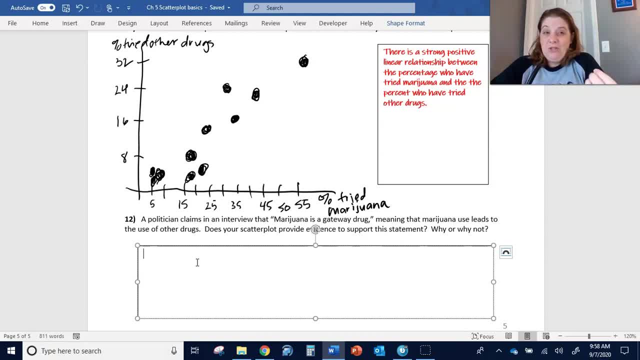 percentage of marijuana users and a high percentage of people who have tried other drugs, And so the percentage of other drug users seems to be high as well. and then low and low. Does that mean that marijuana causes that? And no, it doesn't. Okay, so we would say something like: no, so that. 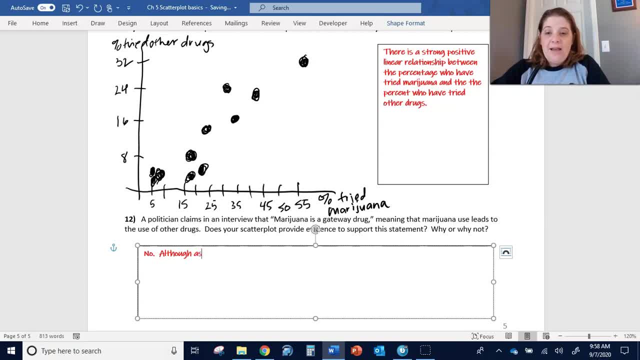 although, as the percentage of marijuana- percentage who have tried marijuana- tends to increase- or sorry, maybe we should say larger values. Okay, so, although large values of the percent who've tried marijuana tend to be paired with large values of the percentage who have tried, 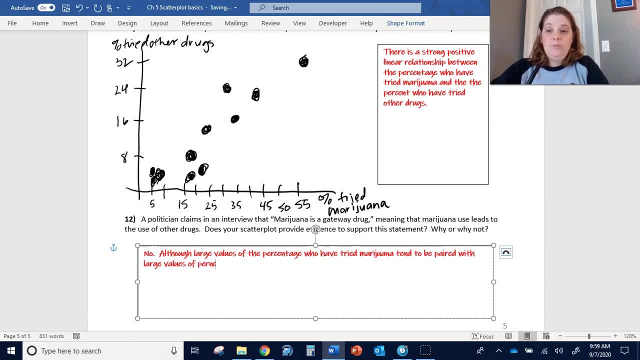 other drugs. this does not show causation. I can't type percentage who have tried other drugs. This does not show causation. This does not mean that trying marijuana causes individuals to try other drugs. So the important thing to remember is: just because you see,